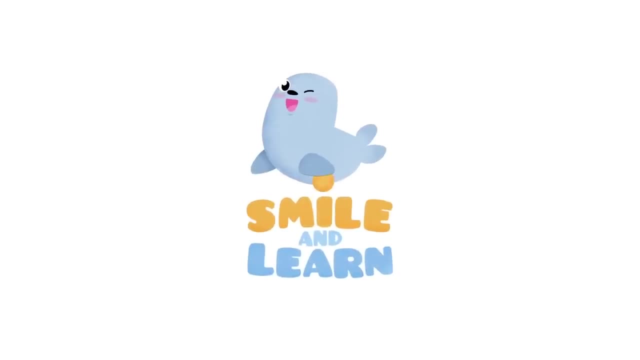 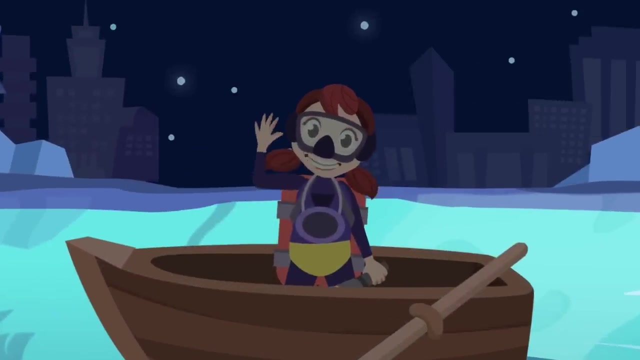 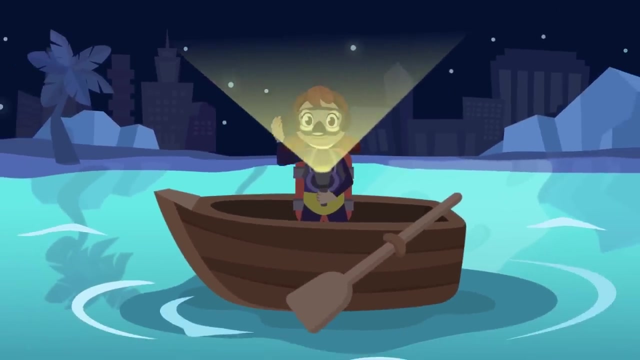 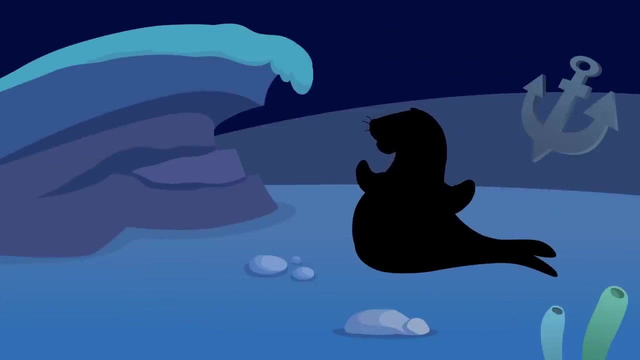 Hello friends, Do you like animals? I love them. Today we're going to learn about aquatic animals. I'll dive in to show them to you. It grew dark again. I'll use my underwater flashlight to find them. I can see something over there. Which animal would that be? 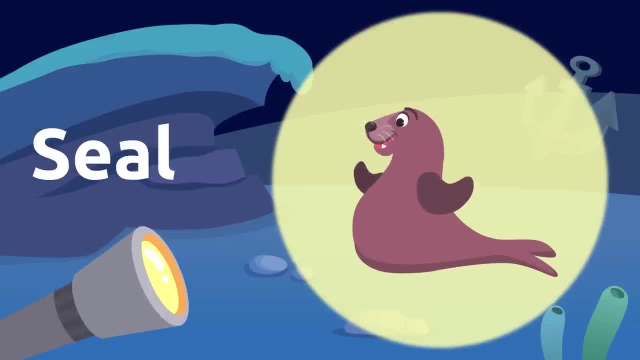 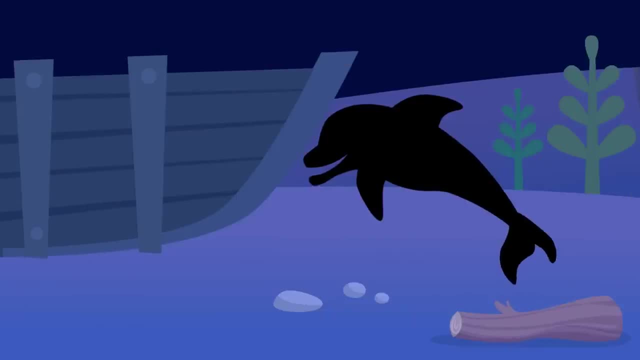 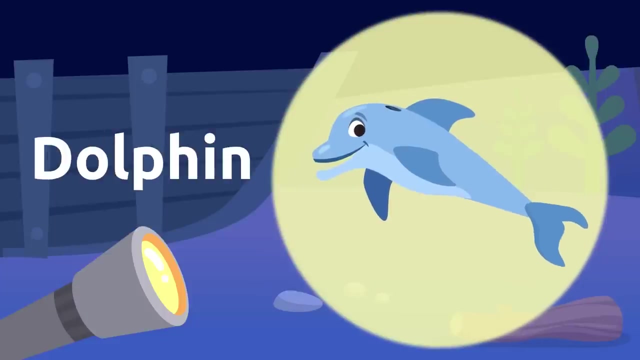 It's a seal Seal, just like the Smile and Learn seal Seal. There's another silhouette over there. What could it be? It's a dolphin Dolphin. Dolphins are very intelligent, Dolphin. What's that animal over there? It's a shark. 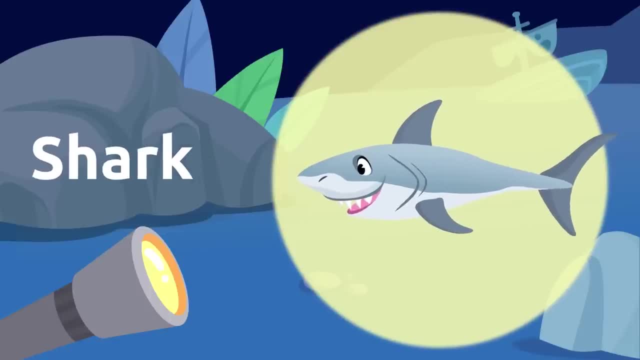 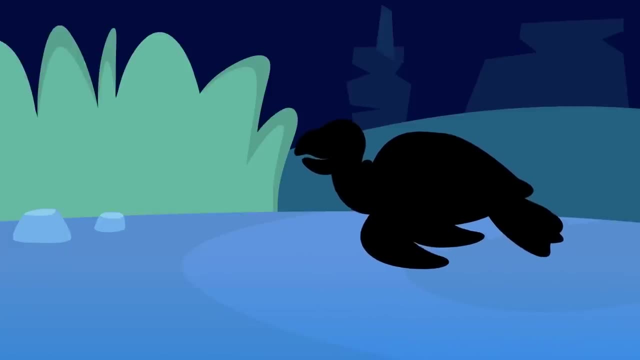 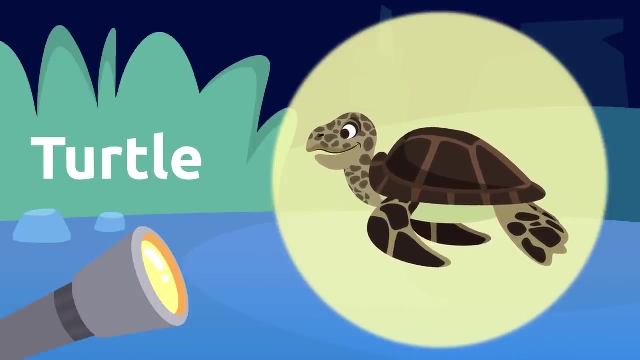 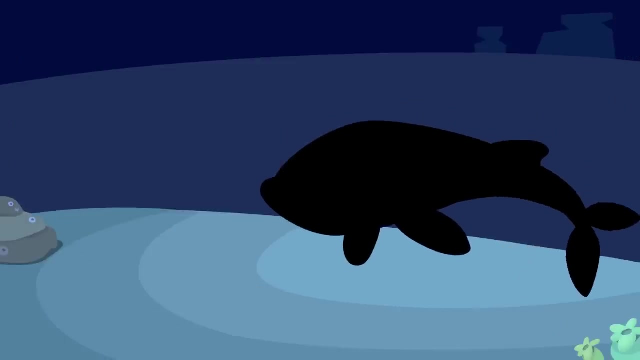 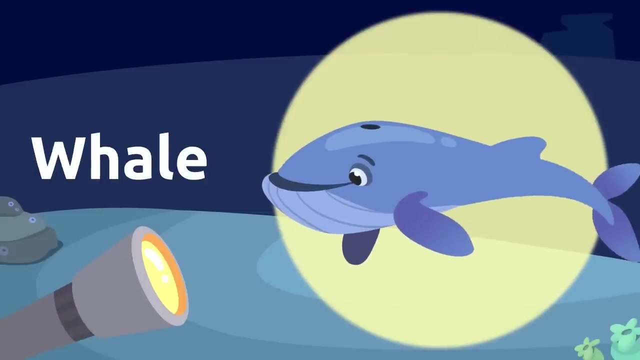 Shark. Sharks are very dangerous animals. Shark, I see something down there. What could it be? It's a turtle. Turtle, Did you know that turtles live many years? Turtle, Whoa, there's a gigantic silhouette over there. I sure know what that is. It's a whale. 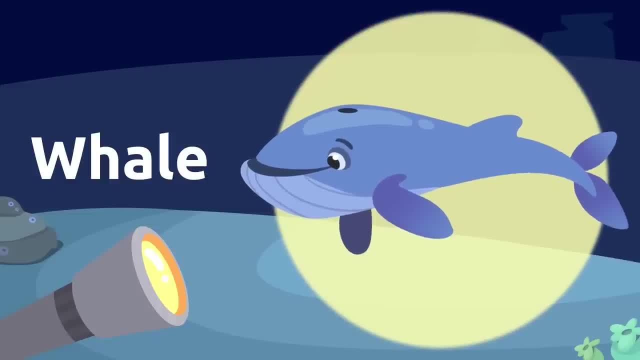 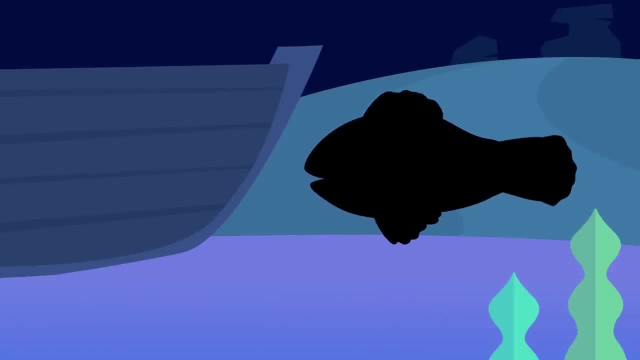 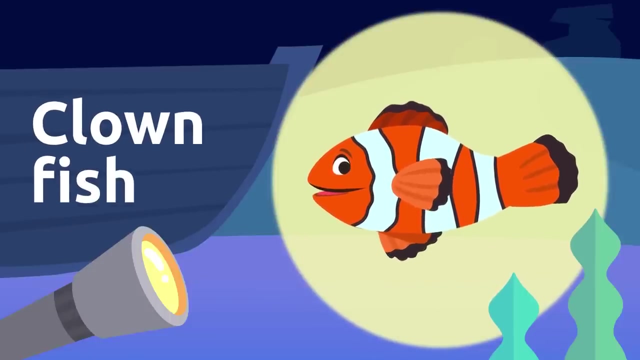 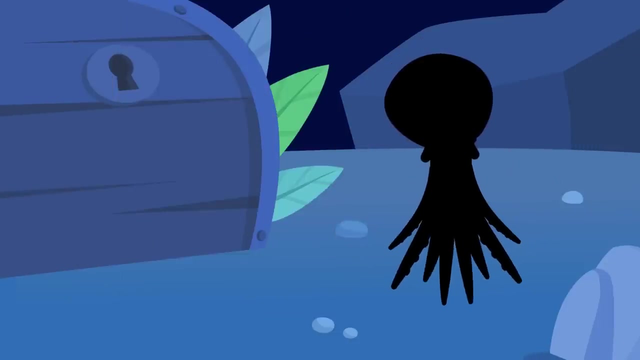 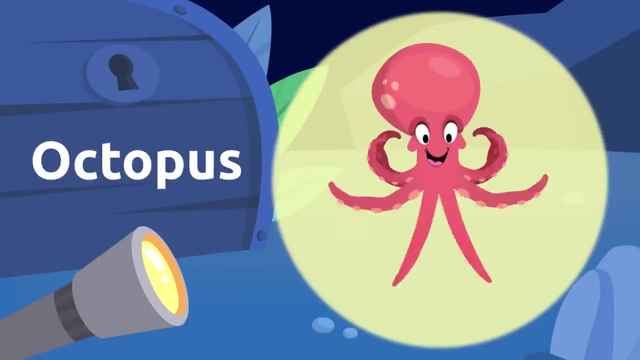 Whale. Whales are enormous Whale. There's something tiny over here. It's a clownfish. Clownfish, I love this type of fish. Their colors are so beautiful. Clownfish, And that weird thing over there, What is it? It's an octopus. Octopus. Octopuses have eight arms. 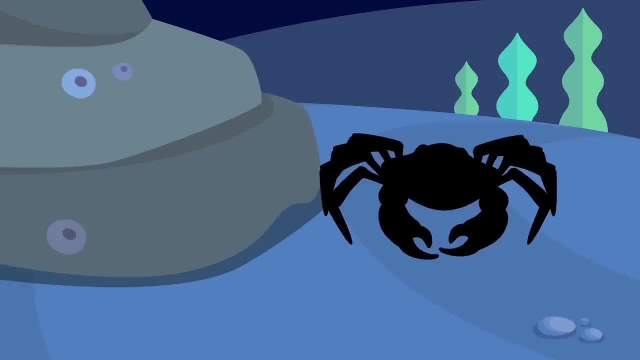 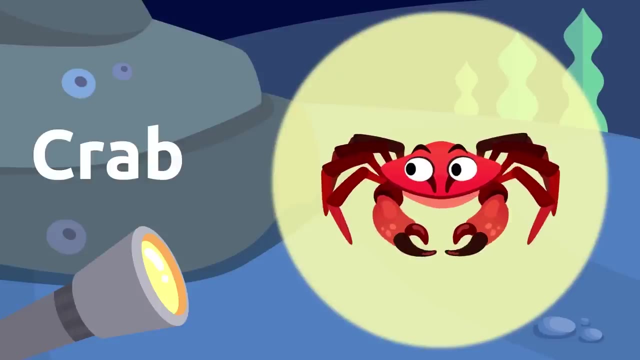 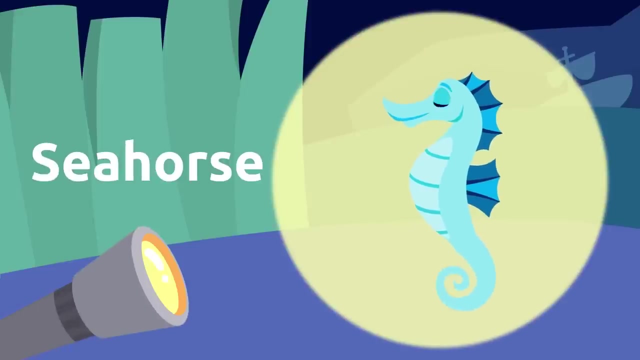 Octopus. There's another tiny silhouette down there. What could it be? It's a crab Crab. Crabs have claws, Crab Crab. What's that over there? What is it? Wow, it's a seahorse. Seahorse. Seahorses are so cool, Seahorse. 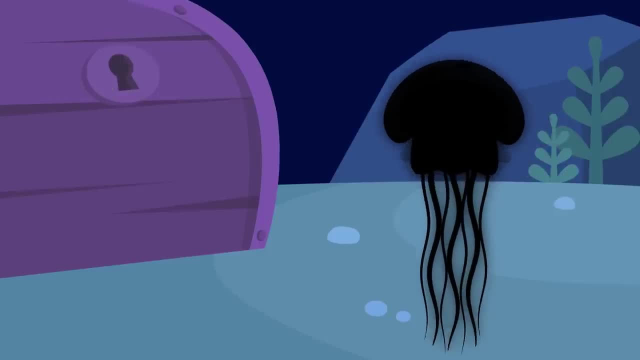 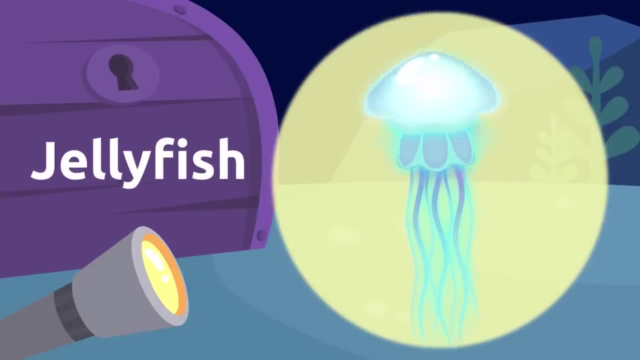 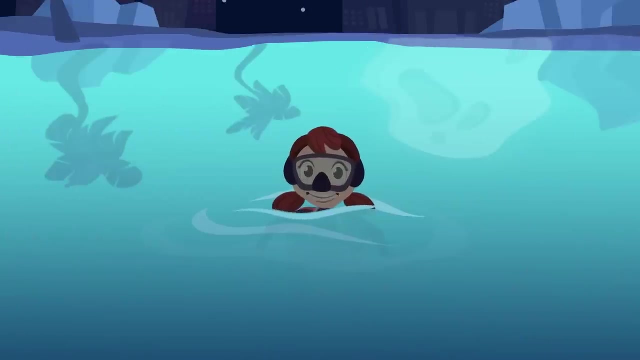 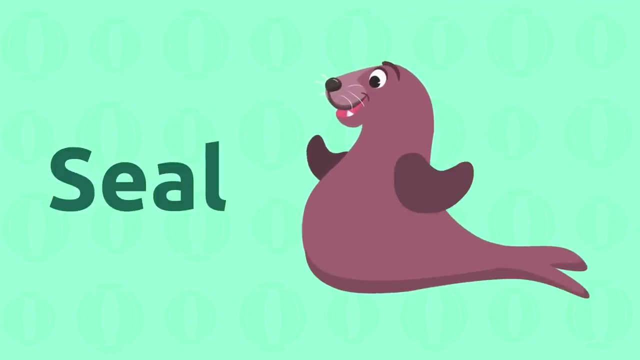 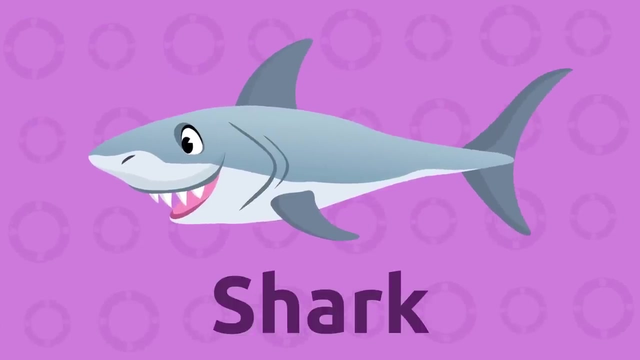 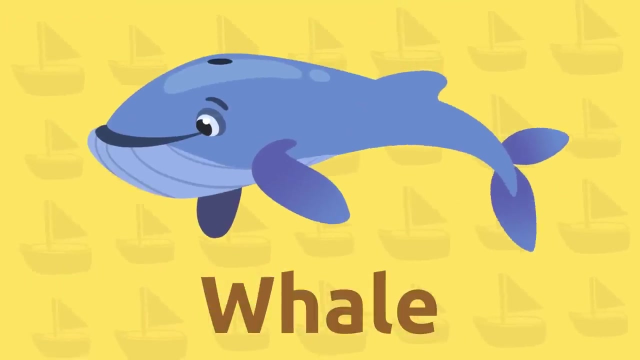 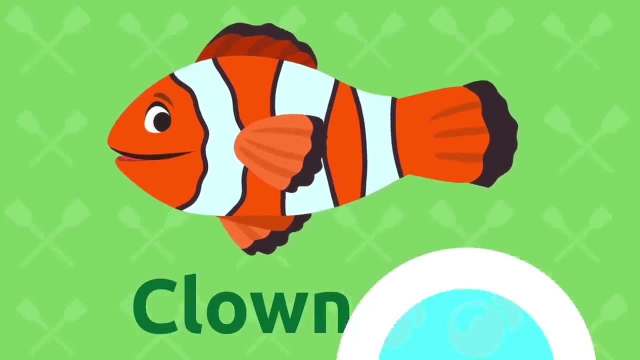 I can see another silhouette back there. It's a jellyfish Jellyfish. Careful with jellyfish, They sting. Jellyfish, Jellyfish, Jellyfish. I can't see any more aquatic animals. Well, shall we recap them? Seal, Dolphin, Shark, Turtle, Whale, Clownfish, Octopus. 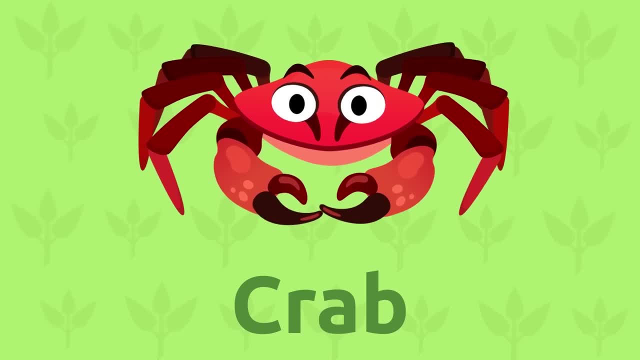 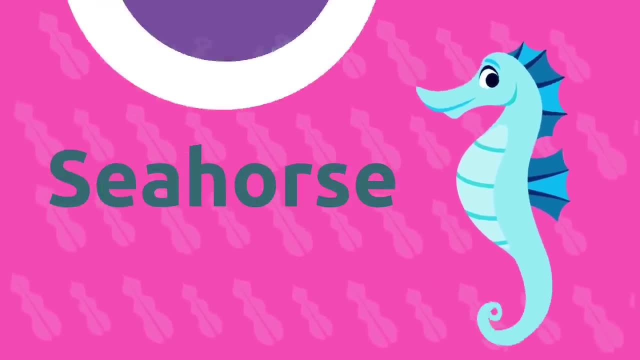 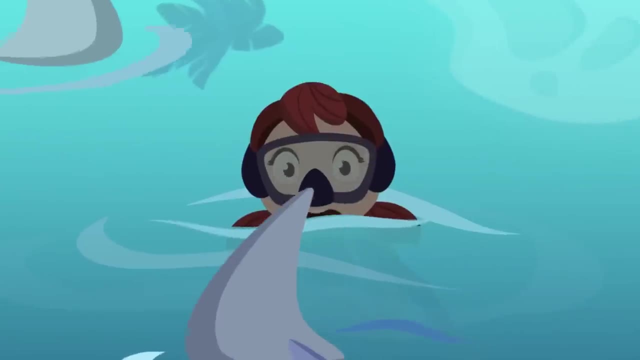 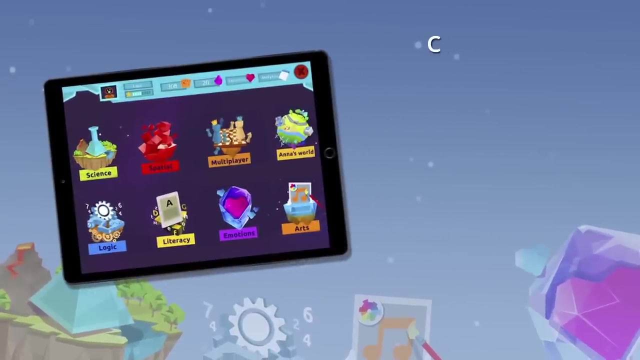 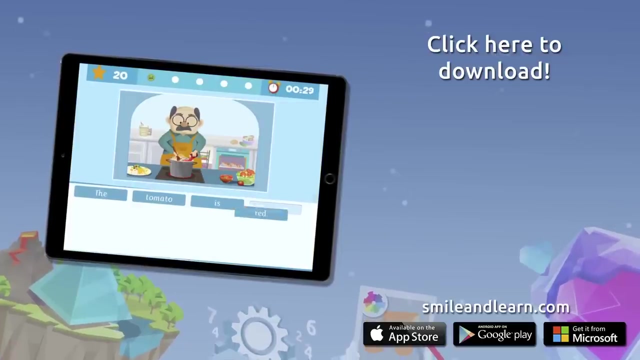 Crab, Seahorse, Jellyfish. I think it's time to get going. Help, Help. Do you want to keep on watching? Do you want to keep on learning? Try for free our Smile and Learn platform for a month and enjoy all of our games, videos and interactive stories. 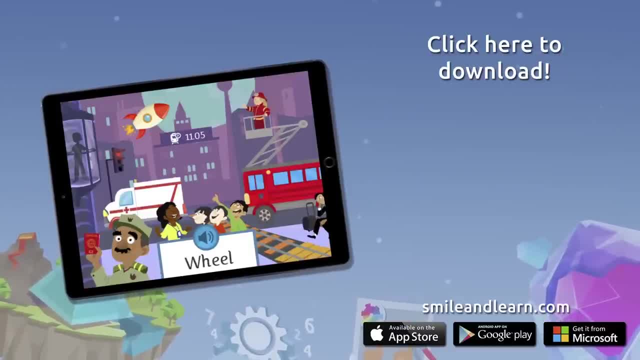 Go for it. Download, Smile and Learn on your mobile, tablet or PC. 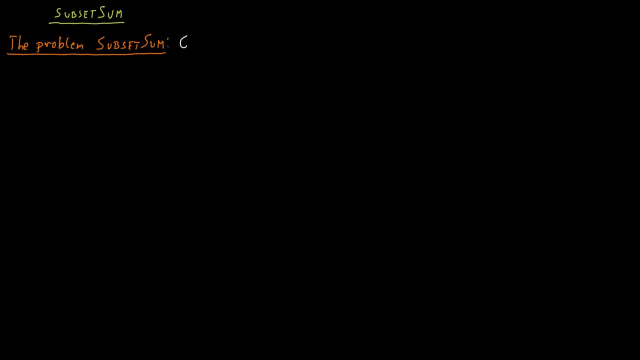 In the problem subset sum we are given n positive integers w1 to wn and an integer capital W. that is sort of a target value, And the question is whether there's a subset of the input numbers w1 to wn which adds up to exactly capital W. So for example, if you 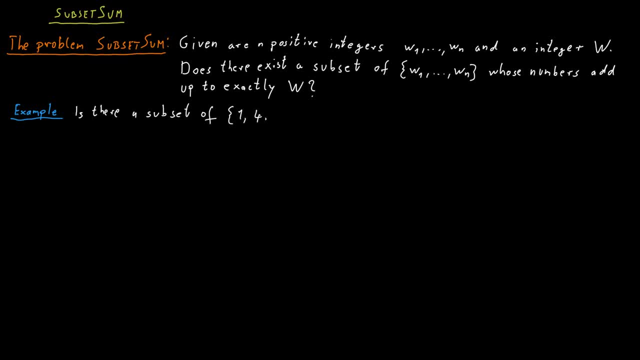 have a set of numbers including the numbers 1,, 4,, 16,, 64,, 256,, 1040,, 1041,, 1093,, 1284, and 1344, and our target value is 3754,, then this is a yes instance of this problem.